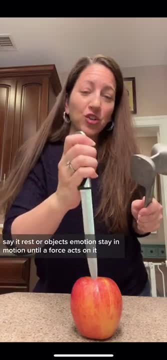 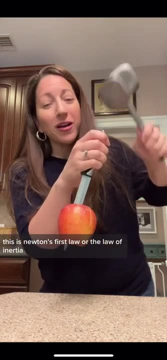 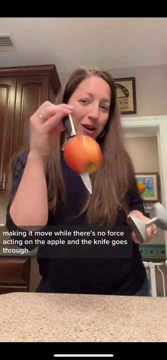 Well, objects at rest stay at rest, or objects in motion stay in motion until a force acts upon it. This is Newton's first law, or the law of inertia. So right now, a force is acting at the knife, making it move, while there's no force acting on the apple, and the knife goes through. So 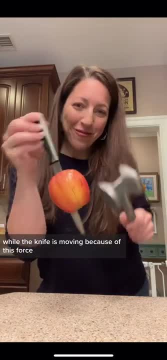 this apple is inertial and it's staying at rest while the knife is moving because of this force. That's physics and that is the law of inertia. Follow for more science, demos. 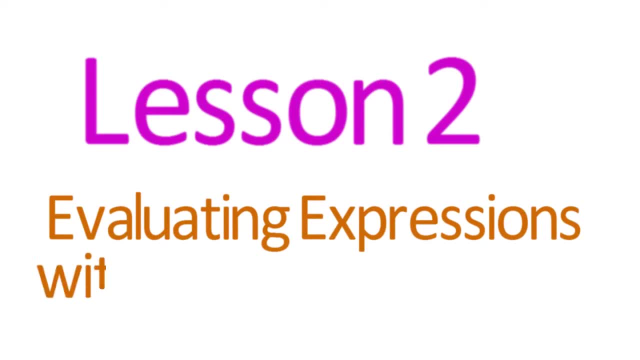 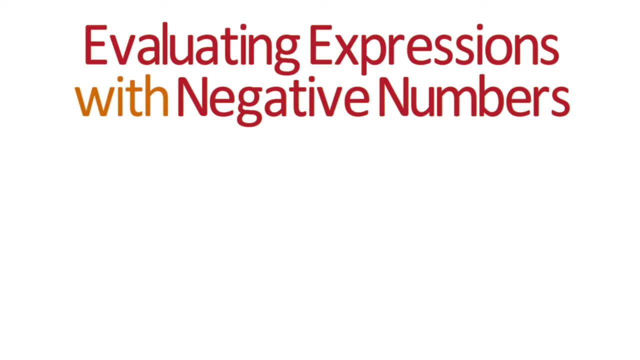 Lesson 2. Evaluating Expressions with Negative Numbers. In the previous module you learned how to evaluate an expression by substituting or plugging in the value of a variable into that expression. This procedure also works when an expression includes one or more negative numbers or when the variable itself is negative. 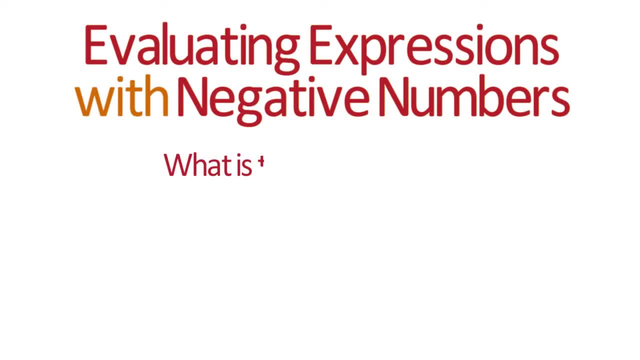 For example, suppose you want to know the value of the expression negative 4 plus k when k equals 6.. To calculate this value, plug in 6 for k into the expression. This gives you negative 4 plus 6.. Now use the rules for adding and subtracting negative. 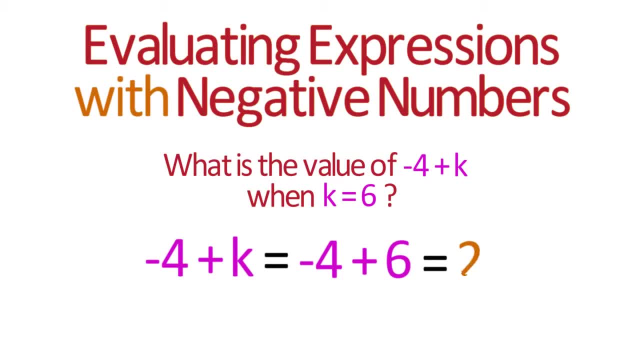 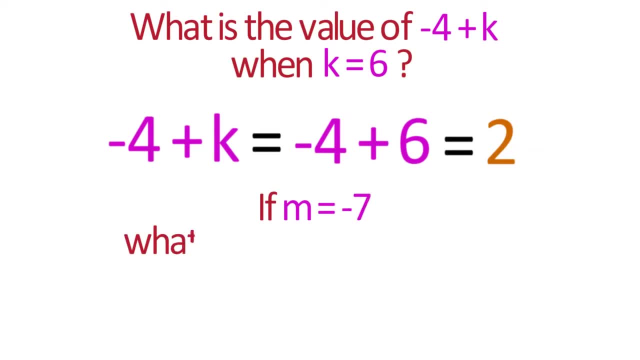 numbers Negative 4 plus 6 equals 2.. As another example, suppose you want to evaluate an expression by substituting or plugging in the value of negative 7.. Suppose you know that m equals negative 7 and you want to find: 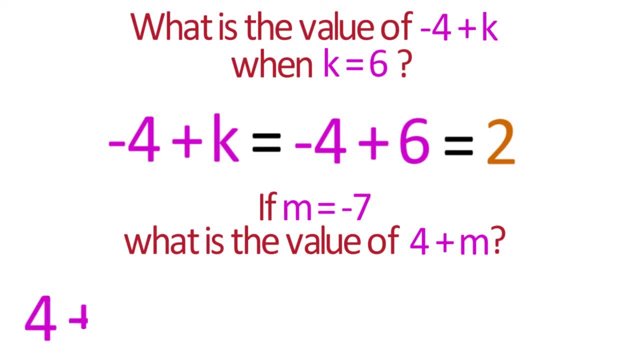 the value of 4 plus m. Plug in negative 7 for the variable m as usual. Remove the parentheses by combining the plus and minus signs into a single minus sign. Now subtract 4 minus 7 equals negative 3.. As a final example, suppose c equals negative 5 and you want to find the 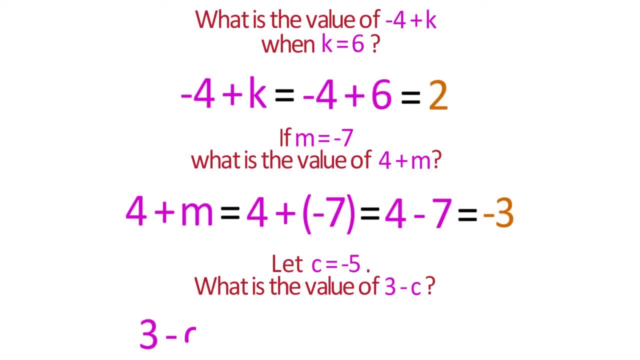 value of 3.. Substitute negative 5 for c into the equation. Remove the parentheses by combining the two minus signs into a plus sign. Now add 3 plus 5 equals 8.. As you can see, all of the rules for adding and subtracting negative numbers carry over into algebra when evaluating expressions.